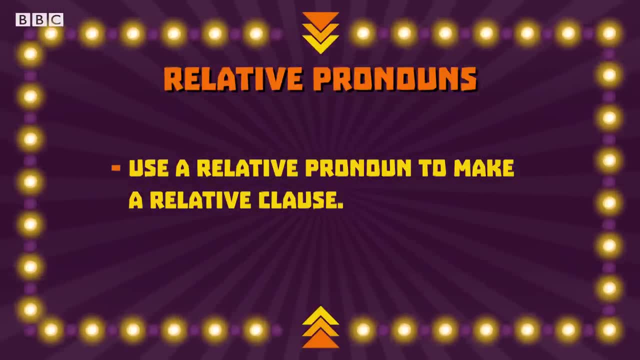 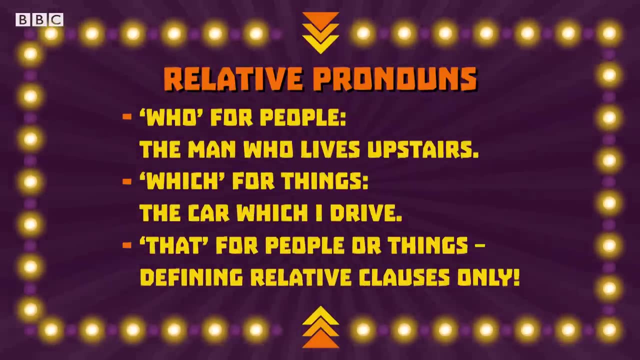 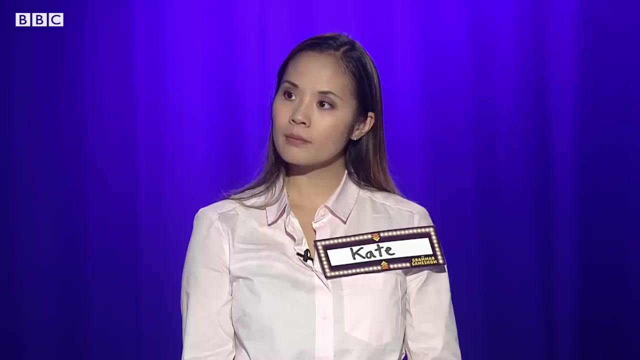 They use the relative pronouns who and which. Who is for people and which is for things. However, in this type of relative clause, both who and which can always be replaced by that. Just remember it's a bit less formal, Levington. four points for you and Kate. 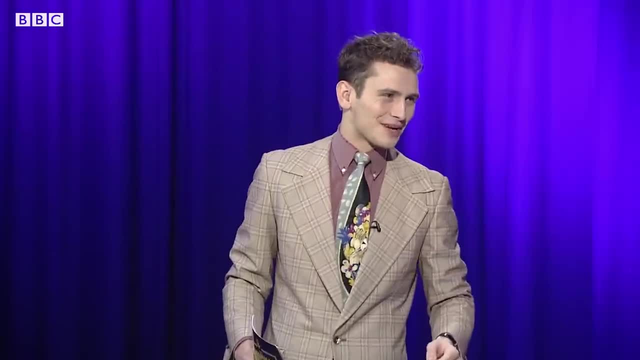 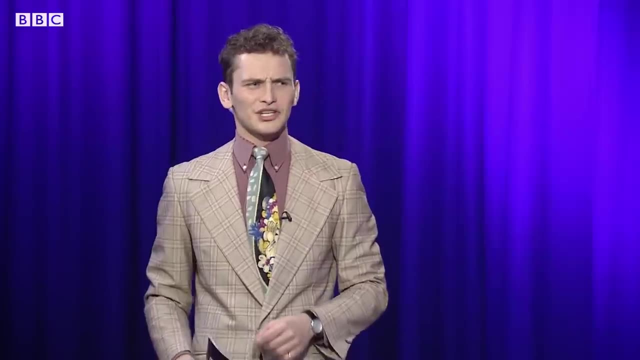 It's ladies night at my favourite club, so eight points for you. Why is that important? Oh, Levington, I see chivalry truly is dead. I suppose you don't give up your seat to a lady on the bus either. 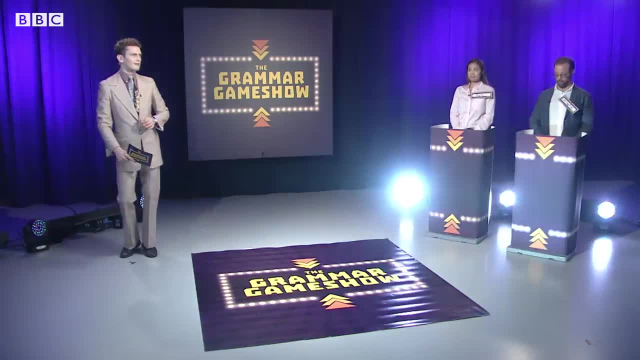 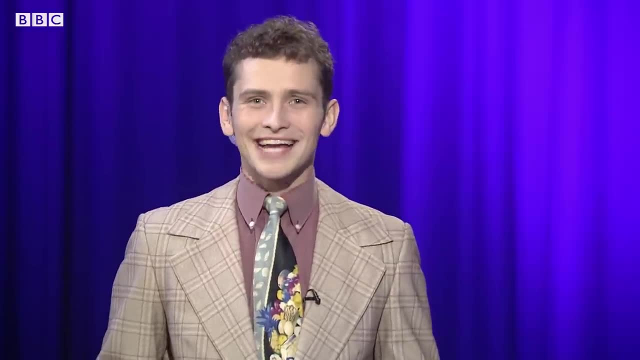 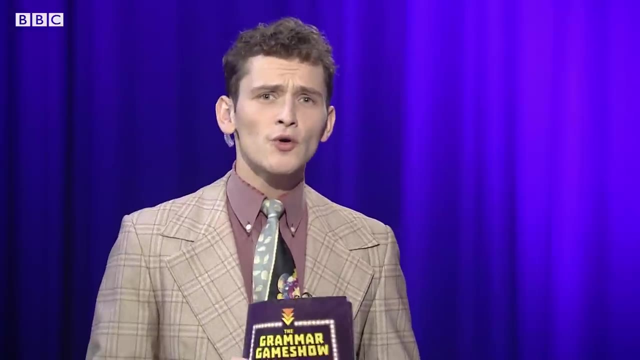 Minus two points for you, No, no. Question two: In addition to who, that and which, the relative pronoun whose can also be used. But why is whose different to who which and that? Look at this sentence and tell me. 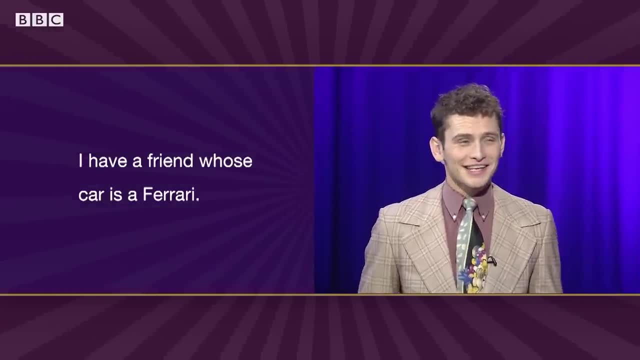 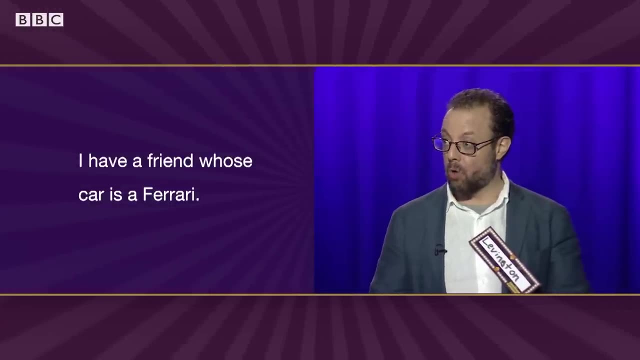 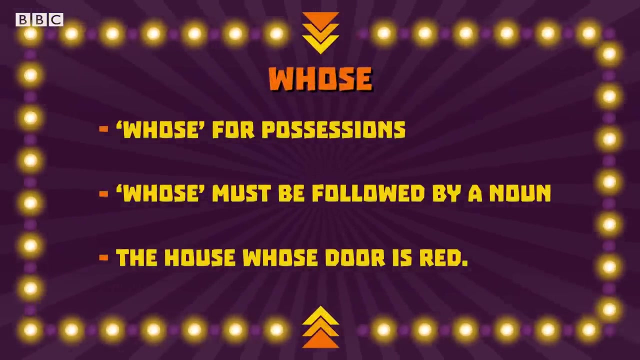 I have a friend whose car is a Ferrari, Whose is different because it describes a possession, Unlike who, which, and that it cannot be used without being followed by a noun- Leslie, Right again Levington. Whose is a determiner like my or your. 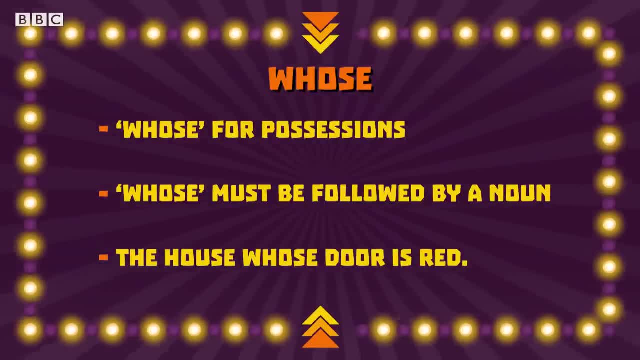 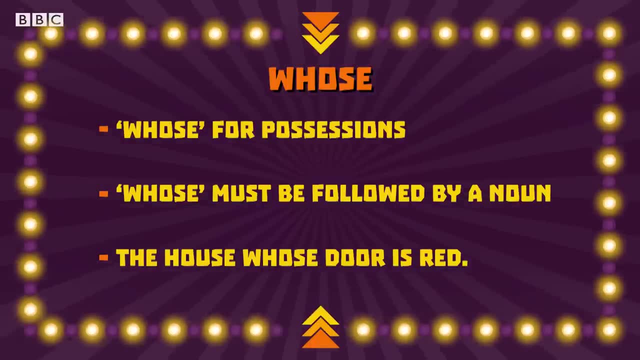 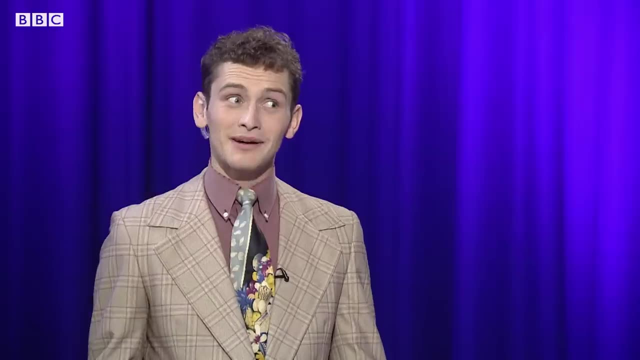 Despite being a relative pronoun, it must be followed by a noun. We cannot say: I have a friend whose is a Ferrari. It must be whose car is a Ferrari. Well done, Levington. However, this is a negative points round. 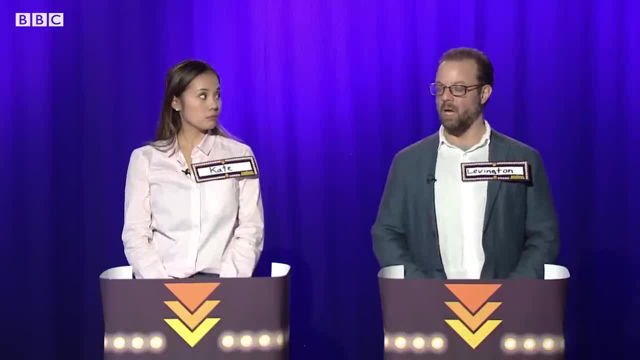 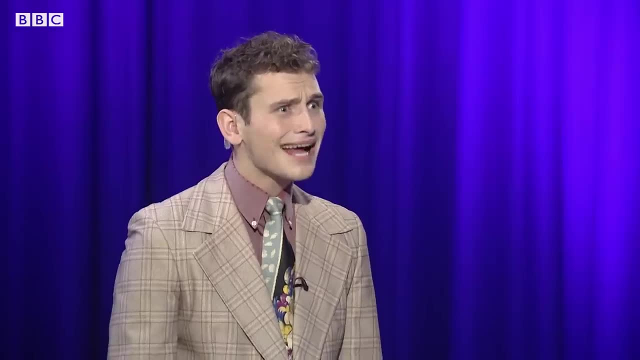 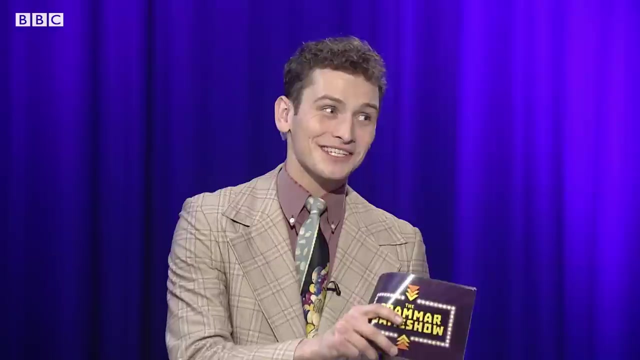 Minus six points to you. Oh, I would graciously like to give my points for this round to Kate. Oh, that's very gentlemanly of you. And because it's ladies' night, all her points are increased. So Kate Levington gives you 100 points. 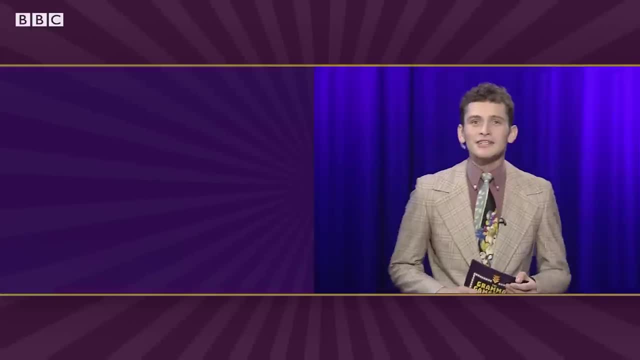 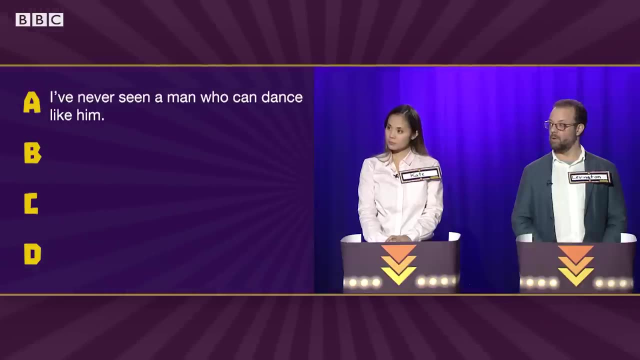 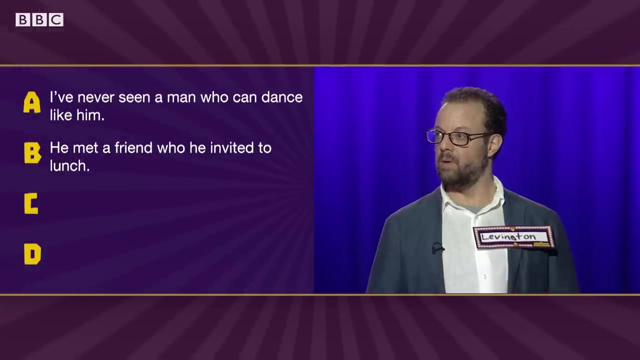 It's time for our last question. Look at these four sentences and tell me in which two the relative pronoun can be left out. I've never seen a man who can. He can dance like him. He met a friend who he invited to lunch.